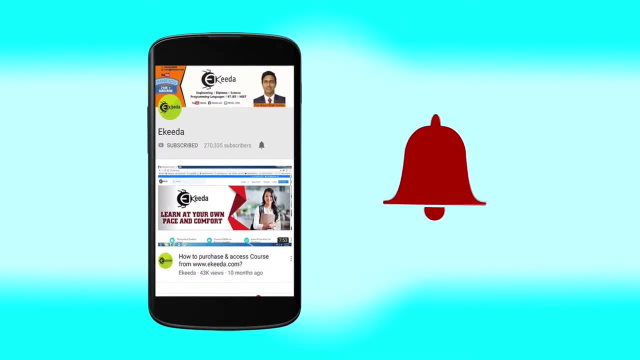 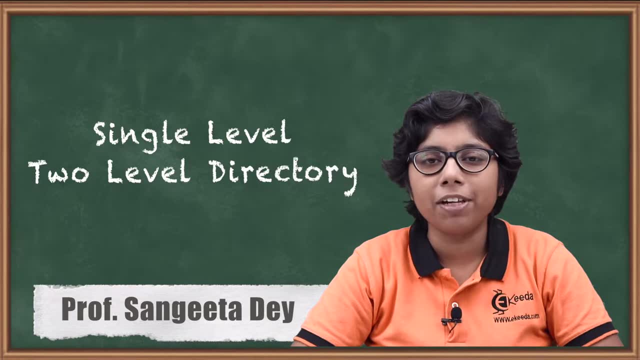 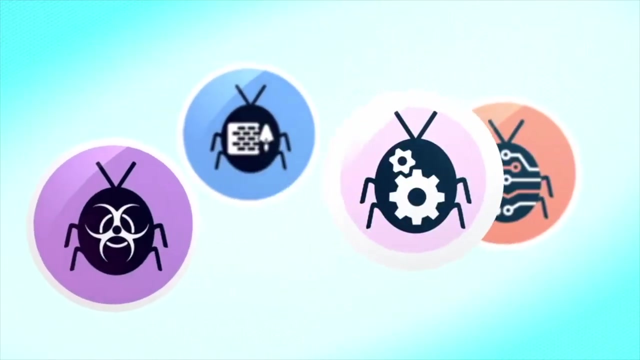 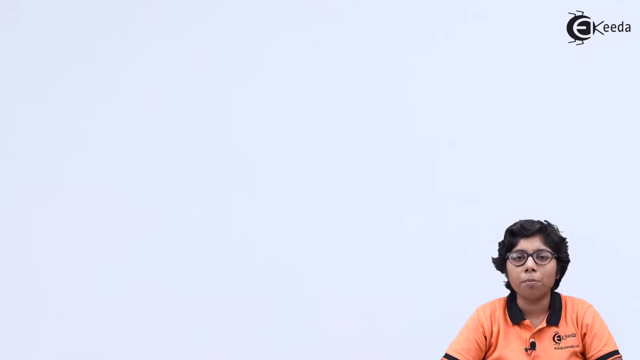 Hello friends, today we will discuss about two directory structures. One is single level, another is two level directory, How this directory structure is implemented and what are the advantages and disadvantages of this particular two level directory structure. Single level directory structure is the most common and simple directory structure used by 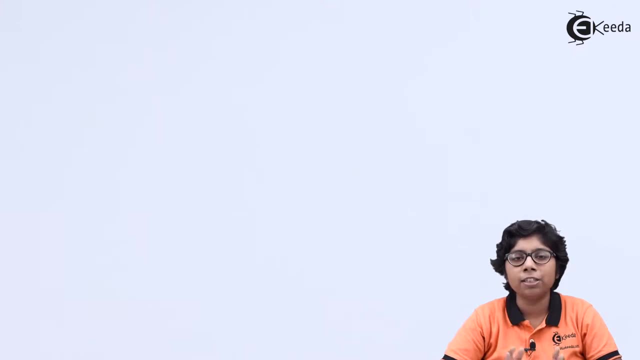 any operating system, It is containing, using the single directory, all the files under it. So whenever an user, or a number of users, wants to refer to their file access, they will search for this single directory and have their files inaccessible, Like when the single directory is used for naming all the files. then two situations can occur with problematic. Number one is the duplicating file problem and number two is the number of users problem. If a user is using a particular file name, then it is possible that other user is also using that particular file name. 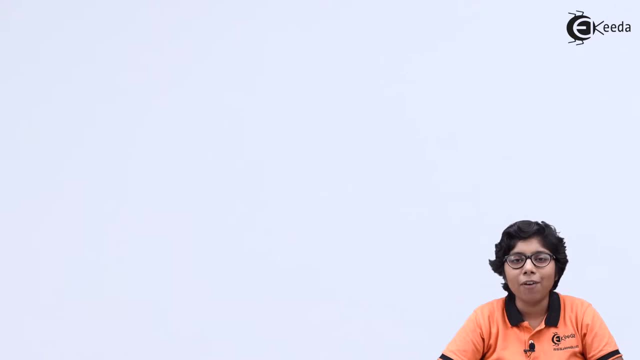 Now to have two users concurrently using the same file name is a problem. under the single level directory, Say, for example, a programmer is used two different task to group sub students. One is 23 number of students, Another is 11 number of students. So the first students groups are using the assignment. 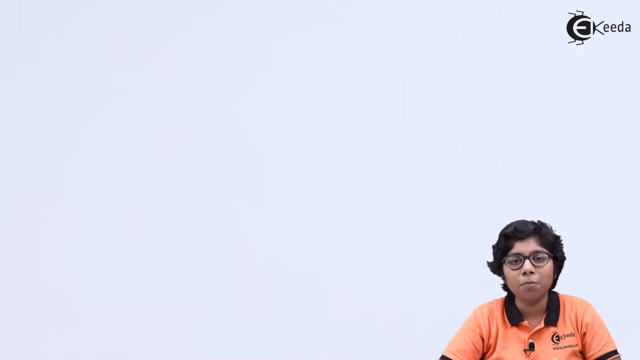 to dot C This file and another 11 number of students is using a probe To see this file. now, as the system supports 1 to 255 characters in the sequence of naming of a file, then it is possible to make a unique name out of this 255 characters combination so we can give the unique name to the 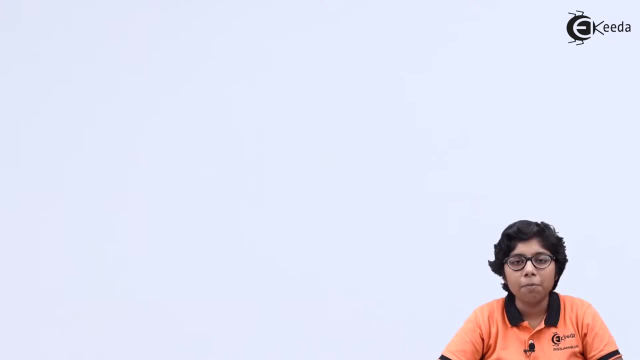 particular file systems. but even with a single number a large number of files become problematic to become in a single directory structure. so single level directory structure that is used for this type of large file numbers can be problematic for a even single level system. now where a single user is accessing a hundreds of files within a computer system, another hundreds. 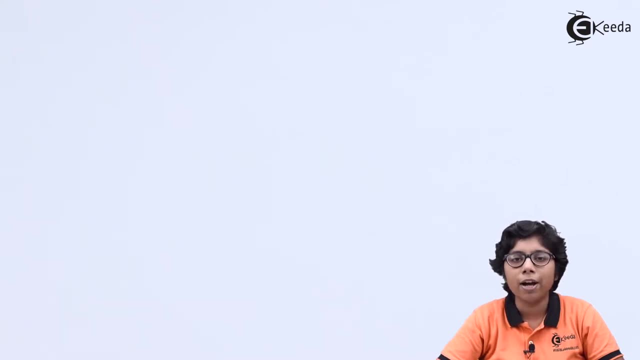 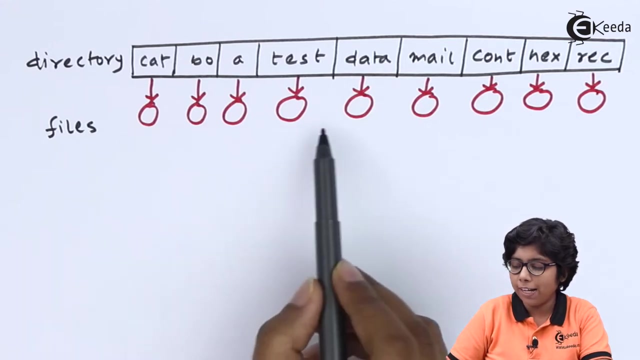 of files within another computer system. so keeping track of this huge number of file system under a single level directory is a daunting task. so we will now see that how, under a single level directory scheme, we are storing the files. so here we can see that all the files that is related to 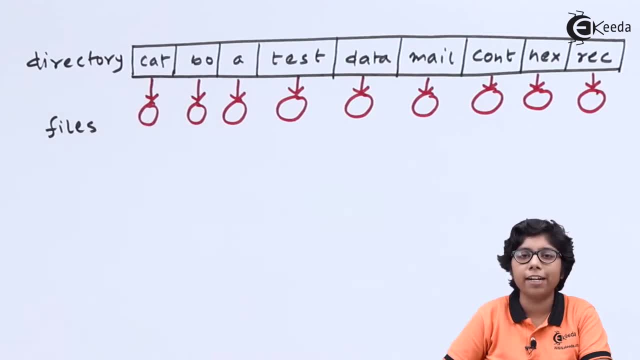 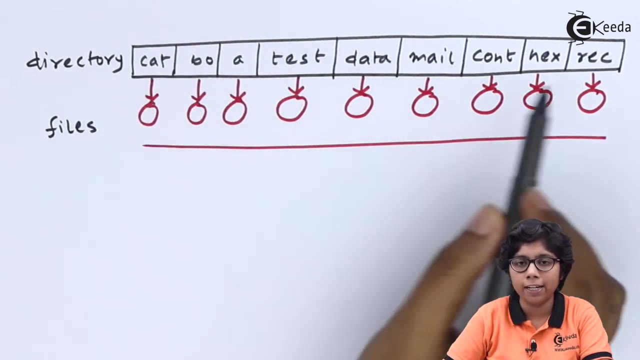 a particular directory is stored inside that particular directory only. now. no files that is similar to a nature then can be stored in different directories. so this is a single level directories system of use, but we can see that the directory numbers are higher as there are many types of files introduced. 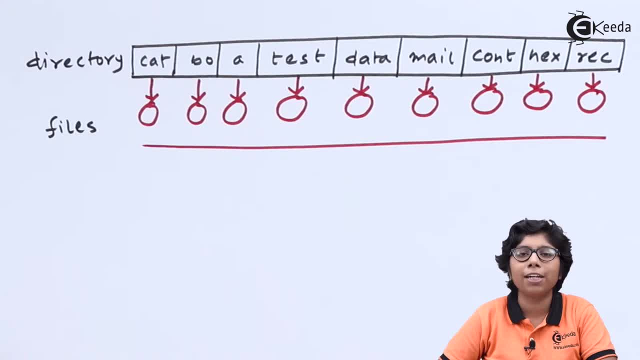 in that particular system. now we will move to the next section of the two-level directory, as we can see that the duplication of num inside a single user or for multiple users is a problem and is a serious problem of single level directory scheme. so to address to this problem we are: 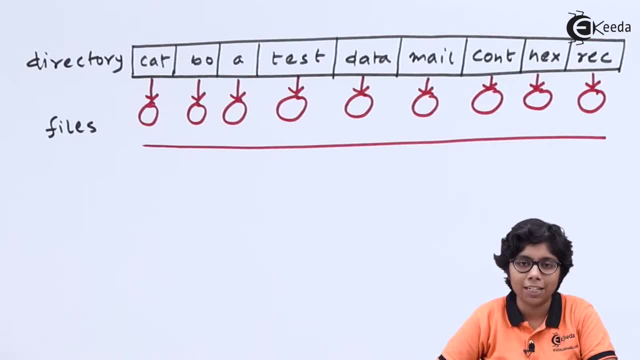 introducing another level of directory that is known as two level directory. in two level directory and user, which is using, all the files are stored inside that user level directory or the UFD. this user file directory is storing all the files that list together full form and operate on that particular user. now 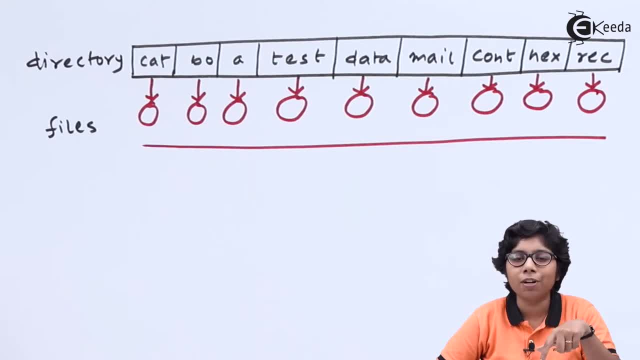 this UFD is a similar in nature, but the only difference is that each UFD can store only the process or files that is operated by that particular user. so when the user logs in or a user job starts, then an MFD or a master file directory. 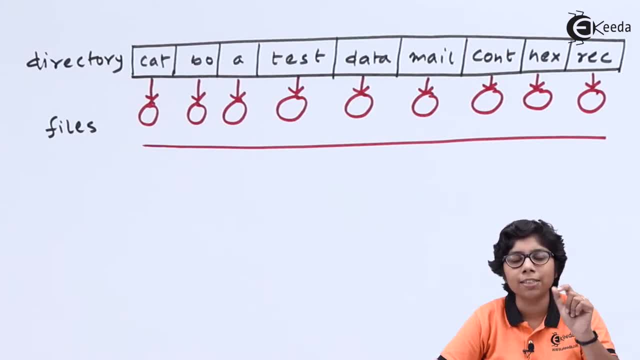 searches for the user process and then locates an identifying pointer to that user process. so it is containing a user number or account number along with fit and a pointer. so it is containing a user number or account number along with fit and a pointer which is indicating to the user process to which that is pointing to. now, whenever 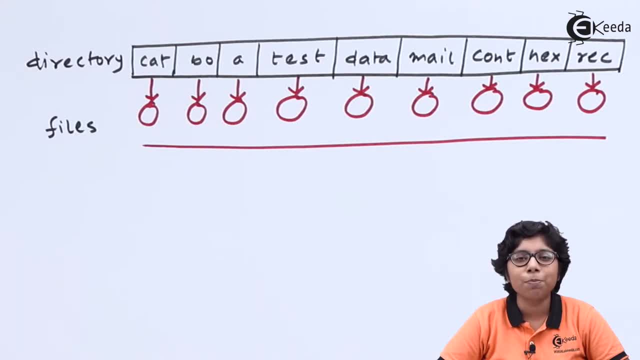 an MFD is pointing to a UFD, then it can specify that how the UFD or where the UFD is located and to locate that file system under the particular UFD. so this clear is very simple. that's UFD is referred for a particular file entered. 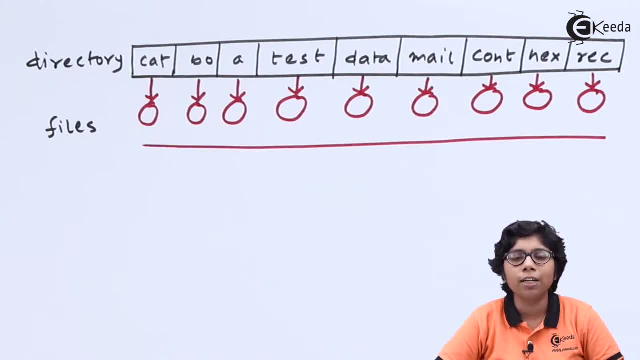 in the process UFD and when a user is running for the system then MFD is searched for that particular UFD. so to search for a file inside this UFD, we need to remember that any name of file that can be duplicated and another number of 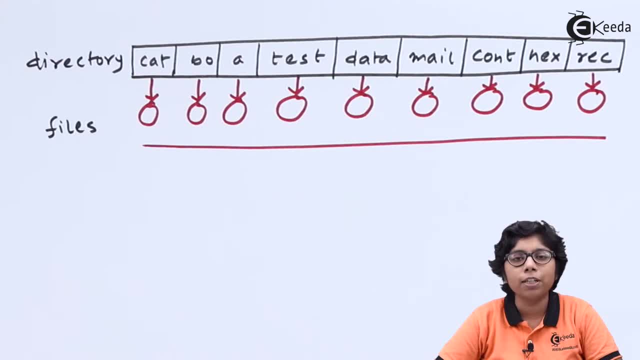 users file in this another UFD. suppose the user 1 is having a file data dot C, user 2 is also can have a file data dot C. where user 1 is not having another file name, data dot C is maintained. so whenever an operating system is creating a file, 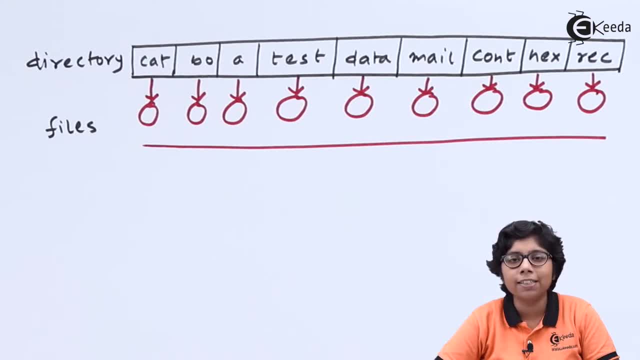 entry in that particular UFD, then it searches that another name of the file is present in that particular UFD or not, and to delete a file, that particular UFD is only searched and deleted for that particular file name. so we will now see how a two-level directory structure actually implements. 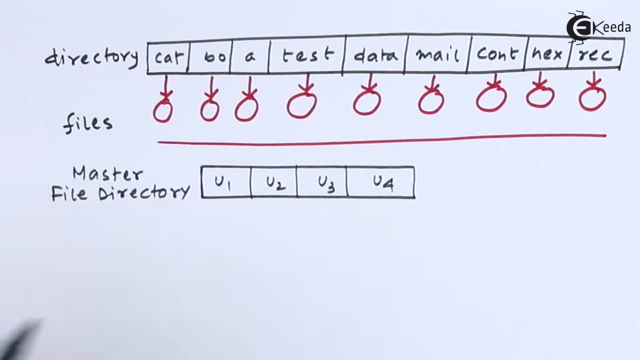 this simple section of your file. so I think we're talking about a directory structure. if an existing directory is not existent in your file, then it will submit all the files that have been sculpted, so we're going to try to separate this state from a directory today. so I've got a county and a. 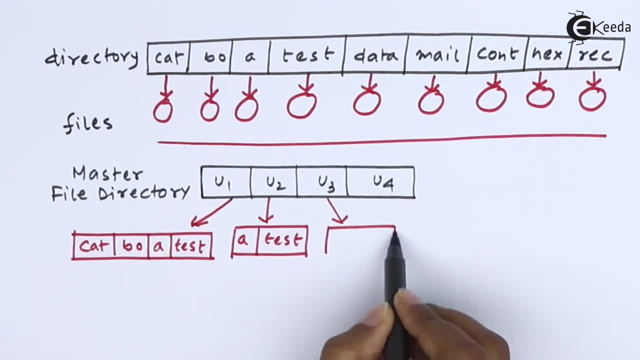 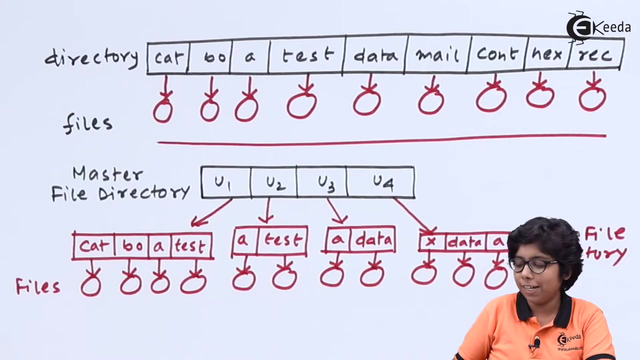 nationality. and of course, the question is if I'm going to put a property here inside that directory. if I don't have a property inside that directory, then I will have to paste the data there. ok, so I'm going to paste the data here. this is so. here we can see a master file directory with four users: u1, u2, u3 and u4. so u1 is having a. 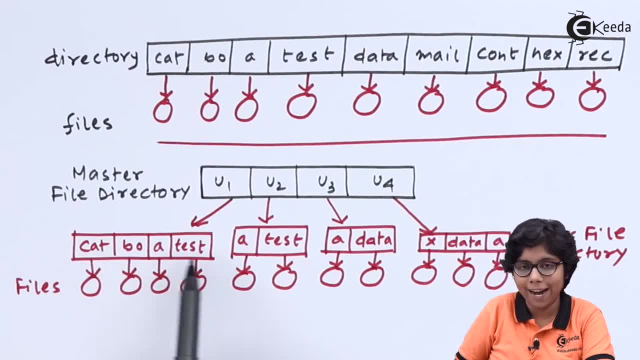 user file directory with the directories cat bow, a and test and u2 is also having the names like a and test. it is common to this a and test, but the files are actually different from each other. the file name can be duplicated but within the each user file directory, no duplicating name. 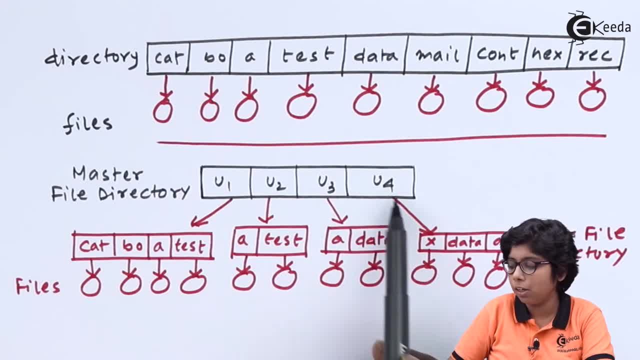 cannot contain. so u3 is containing a data, and u4 is containing data and a, along with another directory, x, and all the directories are containing the actual files in the physical file system. so using this, we can say that this user level file directory and master file directory can make together a two level directory structure. 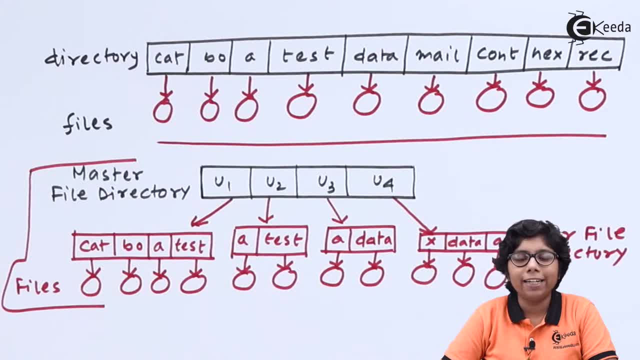 the user directories can be created and deleted as per necessity. now, whenever this creation and deletion comes into question, it is considered as a privileged instruction that is performed by the operating system only. the operating system then creates an ufd on if entry of this u1 and then allocate this entry to the mfd. now this mfd is containing this user file. 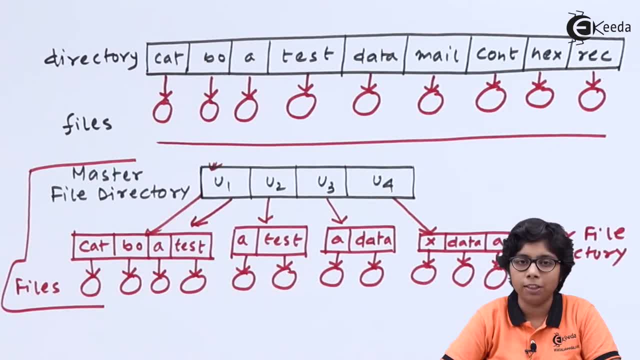 name number along with this pointer to the particular ufd. so the operating system decides that when to create the ufd and add it to mfd and delete for the vice versa. now it asses the duplicated name problem with a single level directory, but it also has some disadvantages. 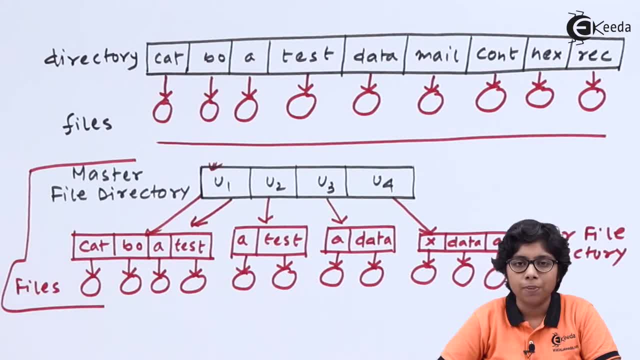 like the problem of the isolation users. the isolation of users is useful when the users that are not cooperating with each other, like each one user, is having their own sets of operation, but if the users are doing a joint work or a group work, then cooperating becomes necessary, and this two level directory isolates these users. 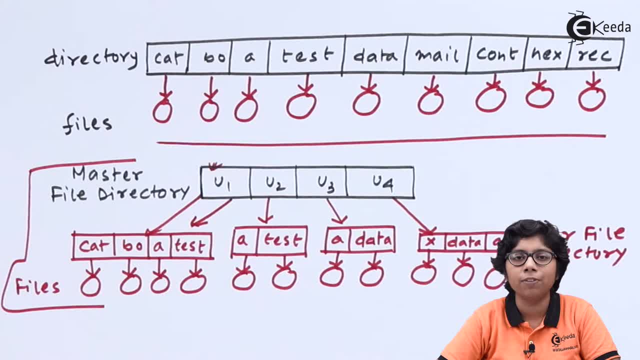 of the cooperating work. so that is a major advantage of the two level directory, as some system do not allow the local file of an ufd to be accessible by another user or another ufd, so the access to get permitted we may want to or we must want to name a file uniquely for that. 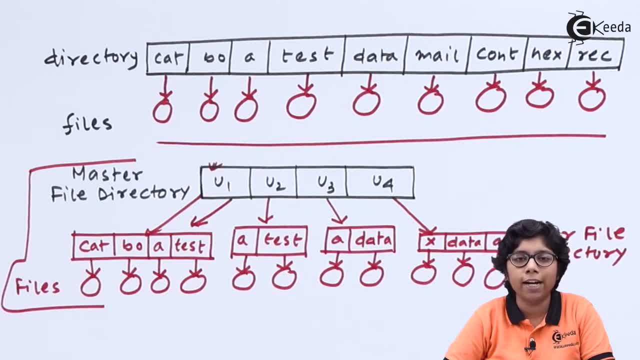 particular ufd or a ufd that is want to get access permitted. so suppose a filename testc is within a new fdu on and another file name, say utu country twp want to operate on that particular file, testc. So it would then definitely make a unique name to that particular file. on U1.. 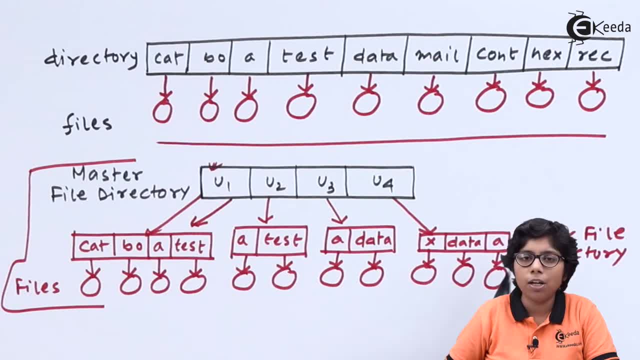 So we can think this two-level directory as a tree of height 2 or an inverted tree of height 2. Where, in the root, we are having this master file directory with the user names and the pointers And as its descendants, we are having the user file directories as their leaves. 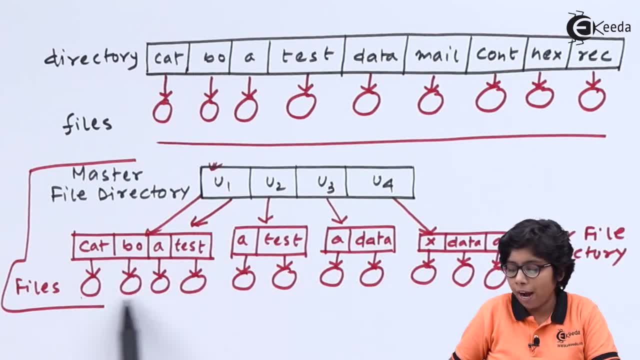 Now this user file directory's descendants are the actual files where the access is made. Now this descendants of this user file directory actually is the leaves of the trees or the final leaves of the trees. So this leaves or the files can be accessed if we make a name: from this root to the leaf, that is, from the MFT via the UFT to the final files. 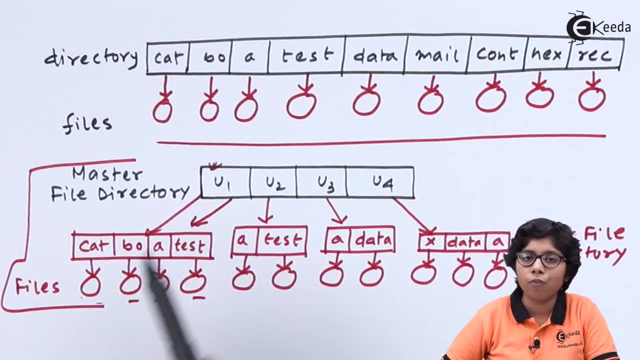 So a path name that is containing from this root to the leaf or from the MFT to the UFT is a name prescribed by the containing all the directory names accordingly or in order. So when you are mentioning the name like So, we are mentioning here that under any user directory, pbj is the directory and testc is the file name. 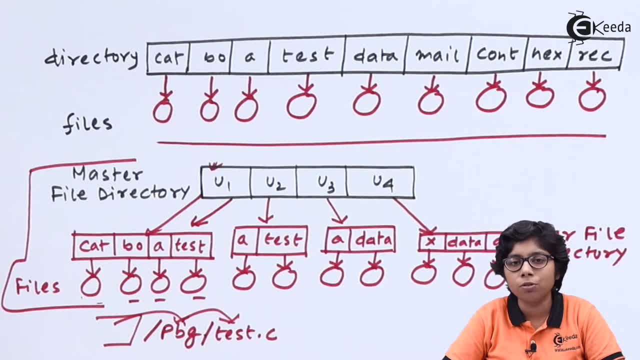 So suppose the user 1 want to direct reference to that particular file, testc, present on its own UFD, So it can refer directly the name testc Now whenever it want to access the u2 file name testdbc which is accessed by the particular u2 user. 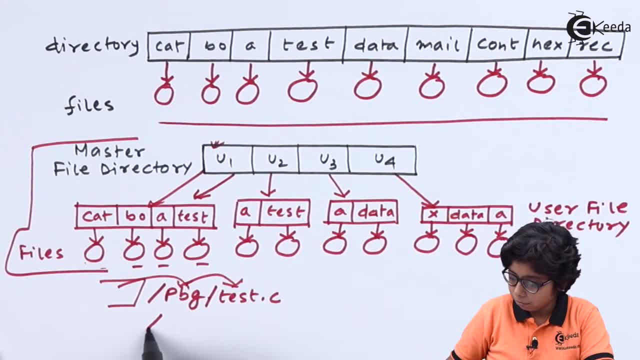 then it should name like where it is mentioning that i want to access the user tools testc function. so this path name is extremely important while the syntax of the memory management or file management of an operating system. so to name a file uniquely, the user must know the path name from the root directory to the 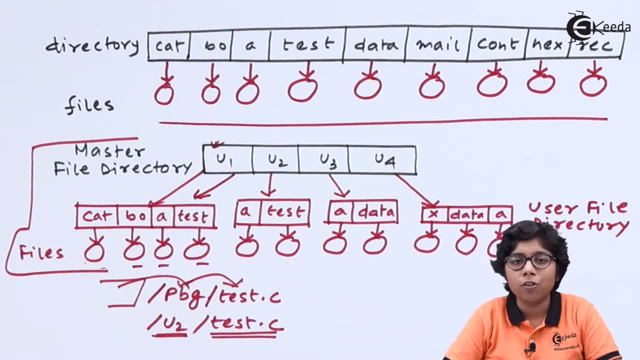 actual files. now another type of syntax or another extension of syntax that is used by the operating system is to include the volume information in that path name. so the path name in windows is generally exemplified with an netter followed by a colon. so suppose, if we are telling like 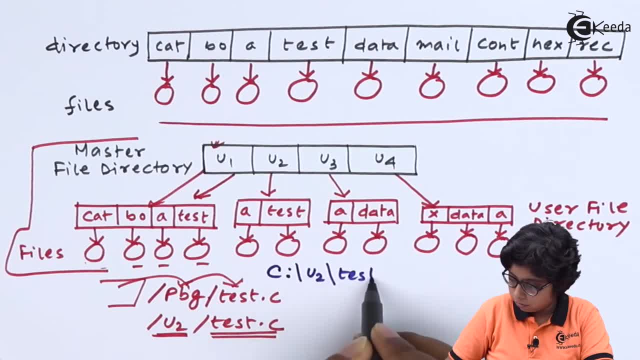 so we are referring here the c as a volume or the root directory u2 as the ufd and testc as the actual file. so now, different operating system uses different types of syntaxes. like unix refers to the volume, information, and another level, to the extreme, that uses that. this u2 must be defined. 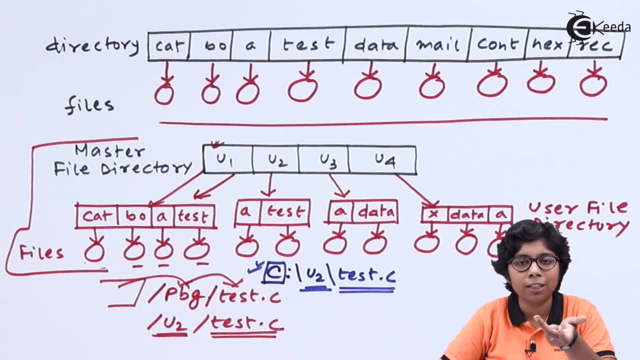 with another bracket and the directory and the directory in the third bracket, followed by the file name. so the exact situation can be described in unix as so here we are using that: c is a volume name, sst is the directory name, u2 is the directory name, testc is the file name, along with a version number of that particular file. 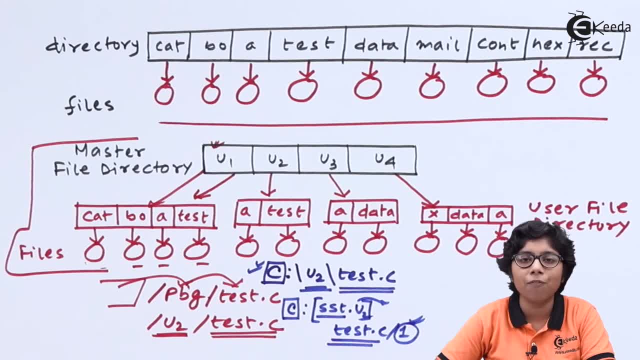 so it can have that the version numbers can be specified to differentiate among the file partitions, like suppose a file having three partitions, one, two, and see, so we can say, test 1, dot C, s to dot C and s 3, dot C has their partitioning. so let is uses the name of the. 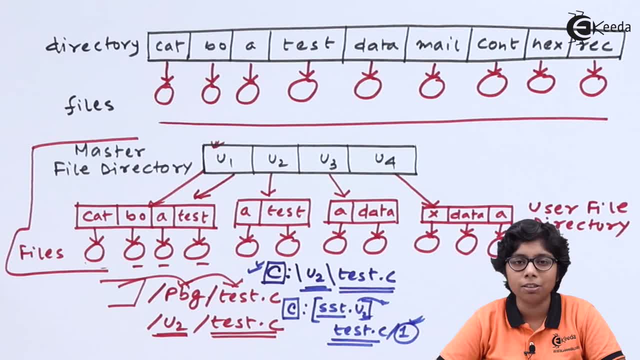 volumes a part of the path name. that is a directory structure. so it uses c, u2, slash, t, stress C as an example of the name of that particular operating system. a special situation may occur in some operating system. now, if you are talking about the system programs, they are often considered as files or normal files. 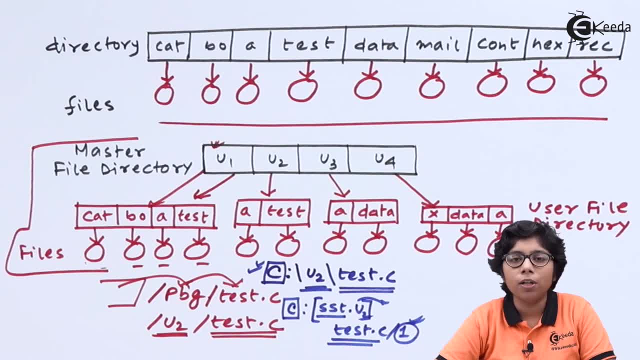 including let this- mfd and ufd. so the loaders, linkers, compilers, assemblers, general routines and libraries are considered as files. now, if you want to access these files, then they should be copied to the each ufd file directory. so whenever we are copying this ufd, it is containing an. 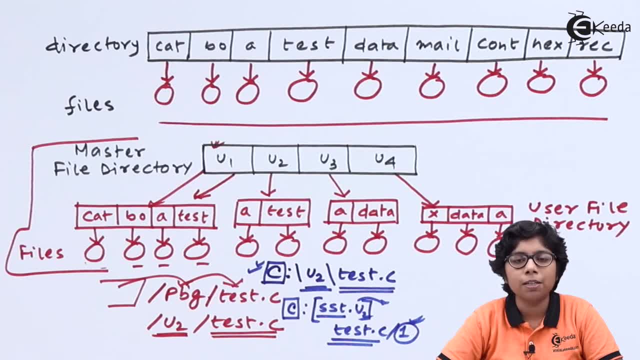 extraneous ordered system. as say: suppose a system file is containing 5 mb and there are 12 users in that system. so 5 into 12, 60 mb of a space will be wasted for just copying the system files. so it is a simple solution to have a system file copy in each ufd, but it makes a 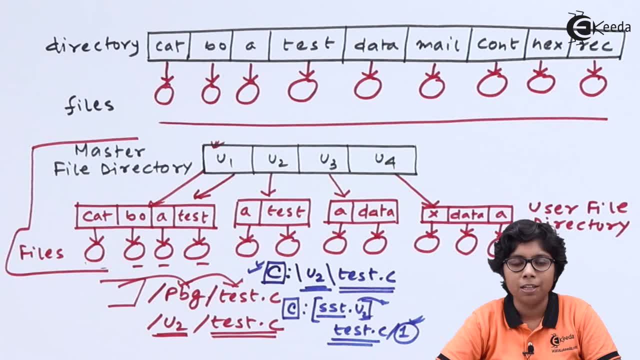 wastage of the memory space by the operating system. so to address to this solution, we can keep a special user directory along with this ufd under a master file directory. so whenever a file name is searched, we can first search to the local ufd. if the file name is found there, it is used. if it is not found, then we can search to the special.